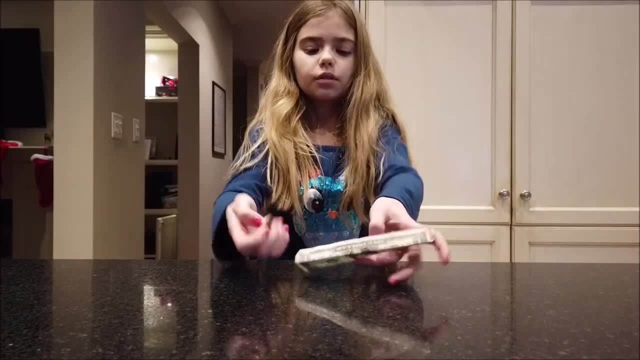 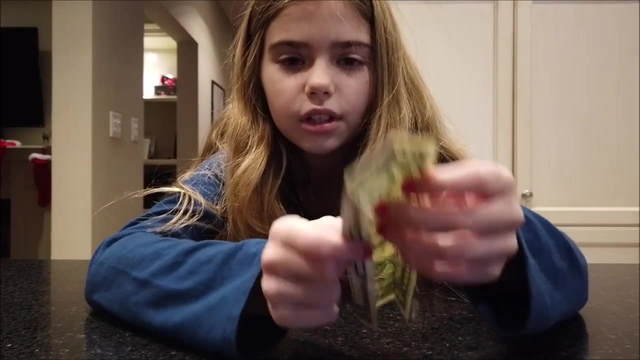 You can also use a maker, You can also use a magnet or something small. So what you want to do, you just want to take your bill and you want to fold down the sides like that. so there's a little room in the middle here. 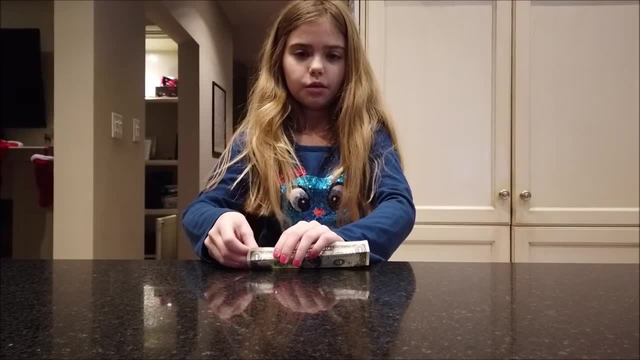 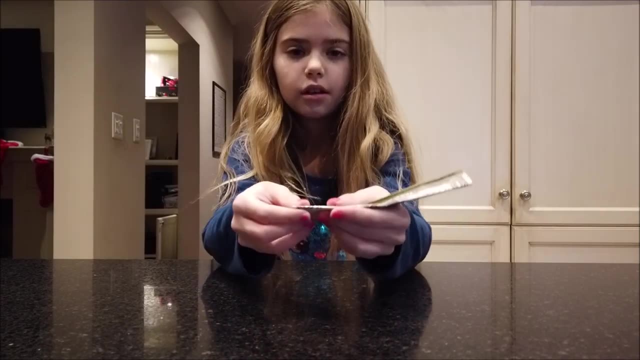 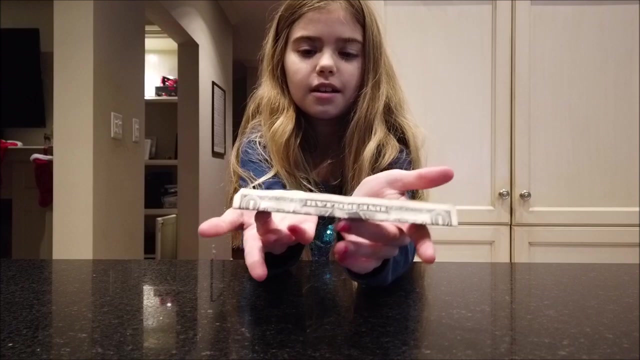 And while you're folding it down and showing your audience, you want to put a coin in and slide it in, And then you just say: I'm going to make the bill float. Put your finger underneath the coin, Go like so And let it float. 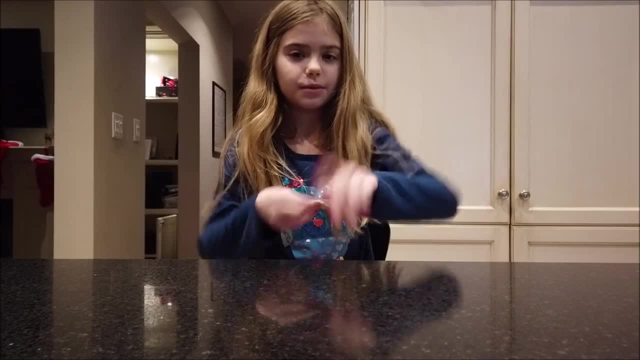 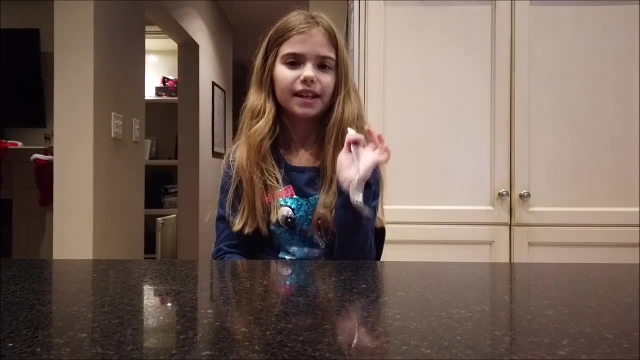 And that's how you do this trick, And let's move on to the next trick. So for this next trick, it's the bending spoon, And you're I mean bending fork. You can also use a spoon if you'd like. 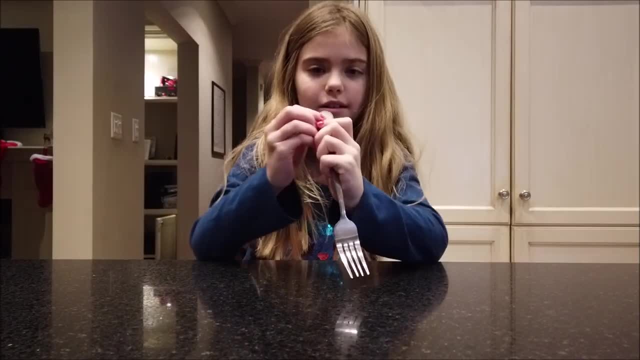 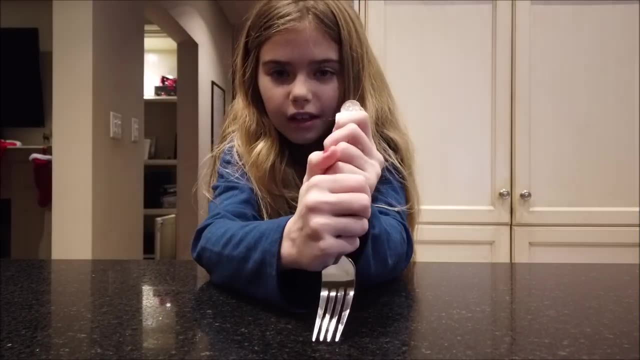 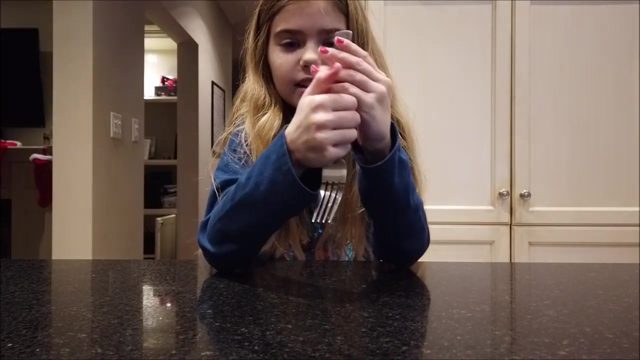 And first I'm going to show you how this should look. So I have like a fork over here And I'm just going to grip onto it And I'm just going to bend it And then bend it back And this fork is fine. 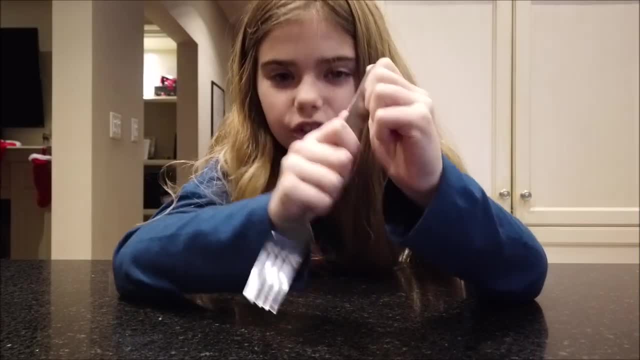 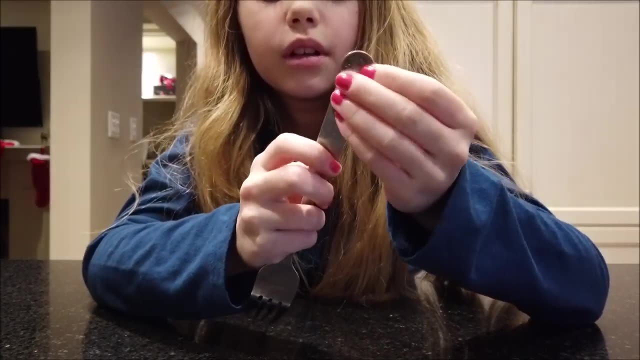 So I don't know if you guys can see, but, um, so you actually need a little coin like this And you want it to be like the same color as your spoon, And you want to do it a bit far away from, like a bit farther away from the person that you're showing this magic trick to. 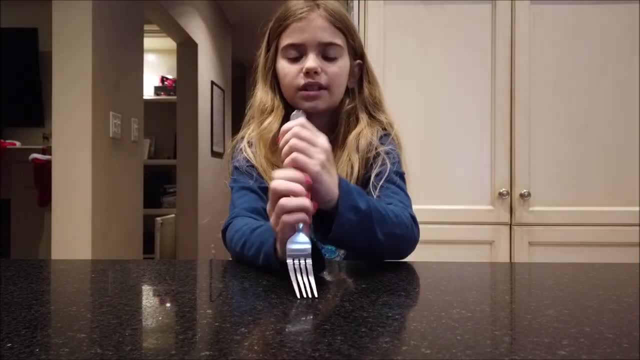 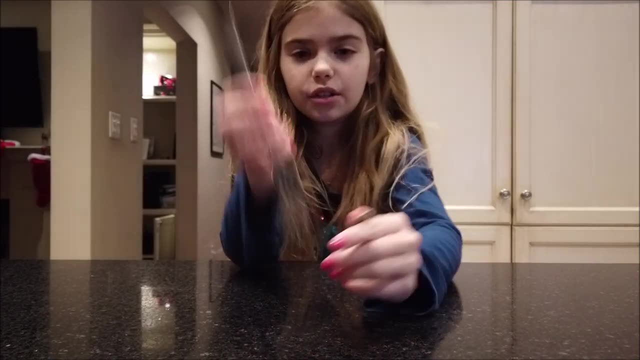 Because you don't want them to see that this is a coin. You want them to think that this is like um part of a spoon And it's bending like this. So what you want to do, you go and grab your fork. 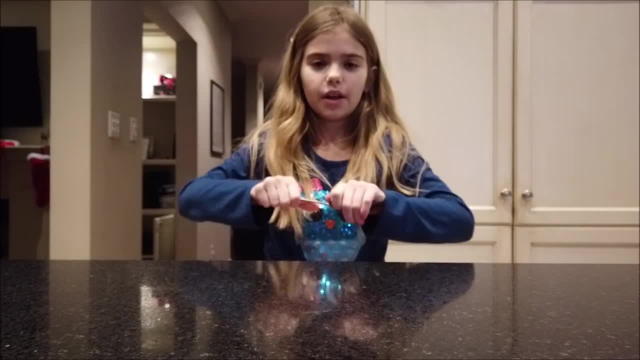 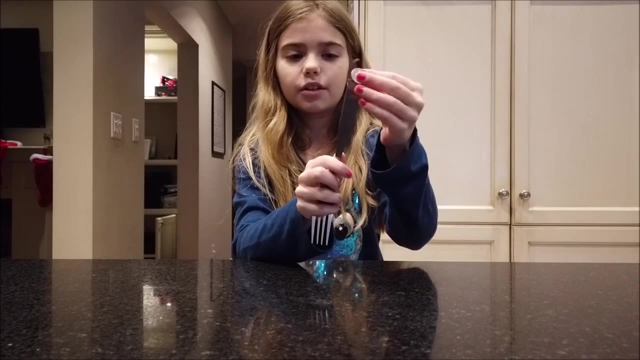 Show it. it's not bending You want. if you want, you can like give it to them and let them try to bend it. Then you just want to go like this: Place your coin here And then just like hold it there with your thumb. 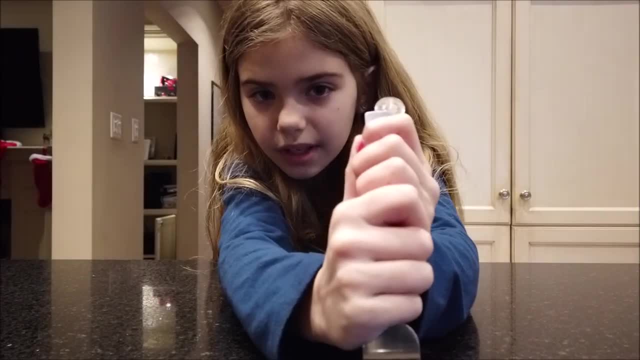 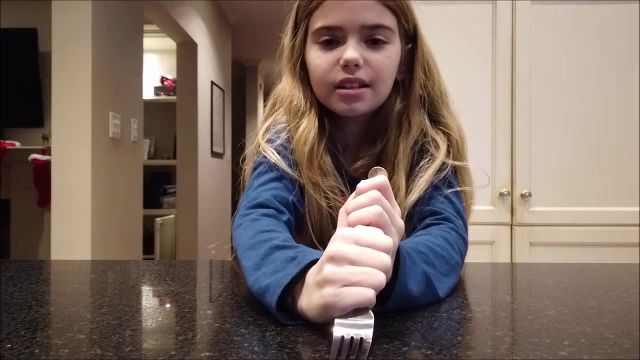 Put your other hand here And I don't know if you can see it, but you just want to like bend it like that, Like keep your coin bended Like that, Go like that, And that's how this trick works. Now let's move on to the next trick. 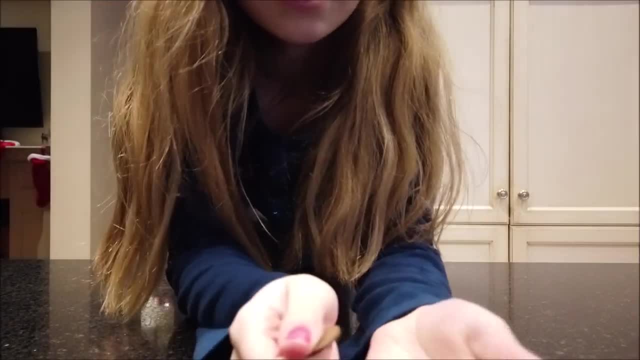 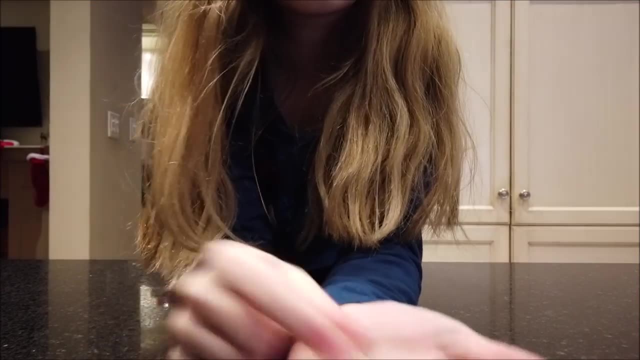 Okay, so for the next magic trick, I'm just going to show you up close, Because I have some um coins here. So what you're? so I have this silver kind of colored coin And this um, this is a penny here.